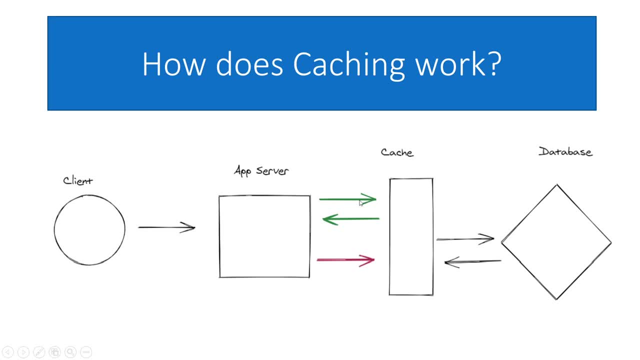 we have our cache. So if you look at in this example, you have a request. If that data is already in the cache, it can serve that directly back to our application, which then sends it back to the client. Down here is: if we don't have that data already in the cache, we have to make a round trip to our database. 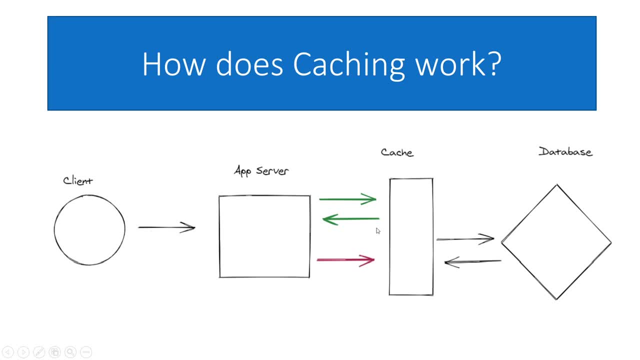 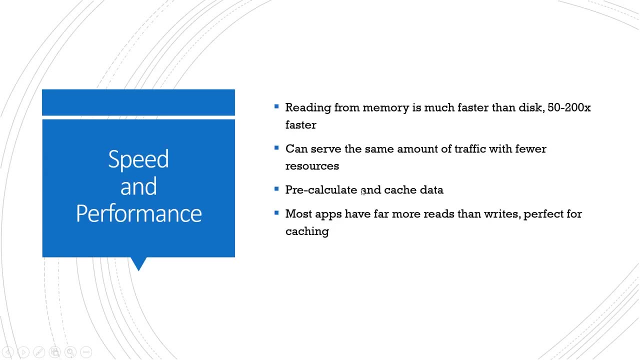 we return it and then we take it back to our app server. So the benefit of this is that delivering that data from cache is much more efficient and much faster. so reading from memory. with cache you're going to see- depending on a couple different factors- 50 to 200 times faster read performance compared to just reading it from. 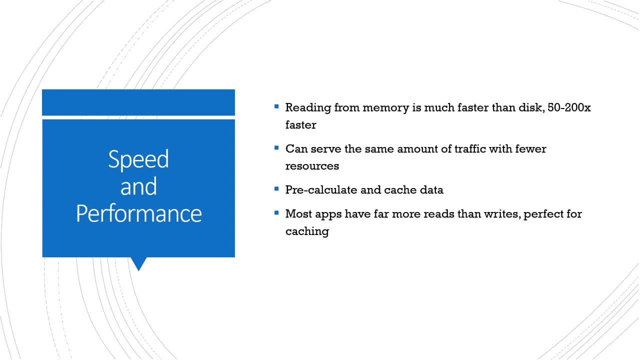 your database. as a result of that, we can serve the same amount of traffic with much fewer resources. just based on simple math of if you're doing something 200 times faster the same, let's say, server with however many gigabytes of memory, it can serve much more, many more requests per second. 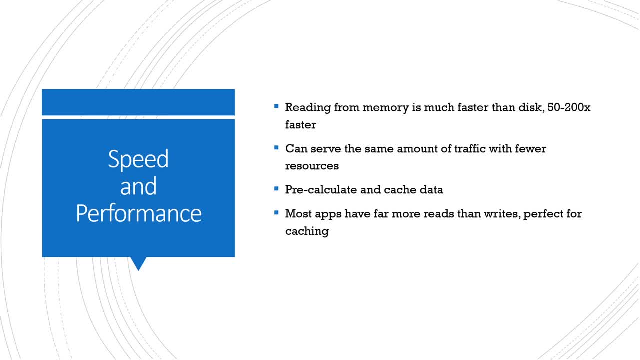 with the same amount of resources. another benefit is that you can precalculate and cache data in advance. so this is something that twitter does with their timelines. they know that users are going to want their timeline very fast, so they'll occasionally pre-compute what your timeline is. so 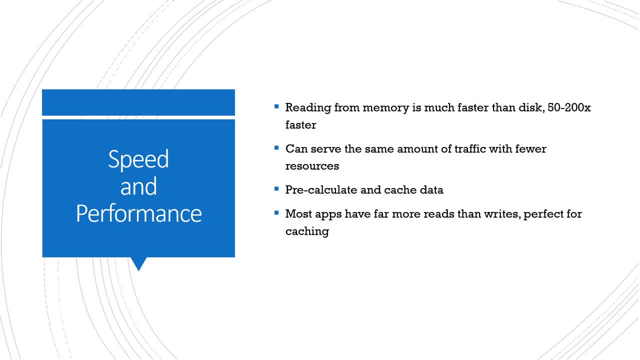 maybe 200 tweets. they'll put it in the same amount of time as ever and then they can pre-calculate it so they can preview it in the same amount of time, so that you can easily pre-compute your that data to cache, and then they can serve it very quickly. so, instead of every time you request. 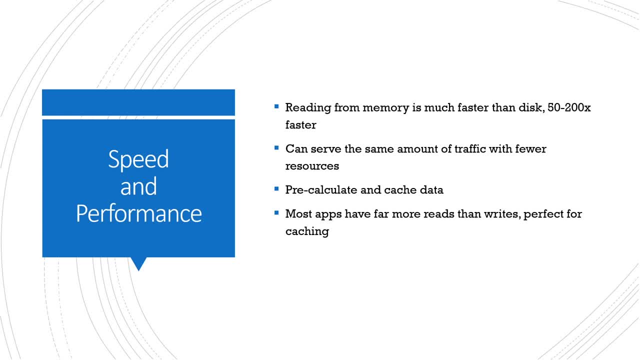 twitter having to go to the database, run their algorithm to get your news feed. they pre-calculate it and they can serve it within milliseconds, rather than a couple seconds waiting for all that to process. so if you know what your users are going to need in advance, you can. 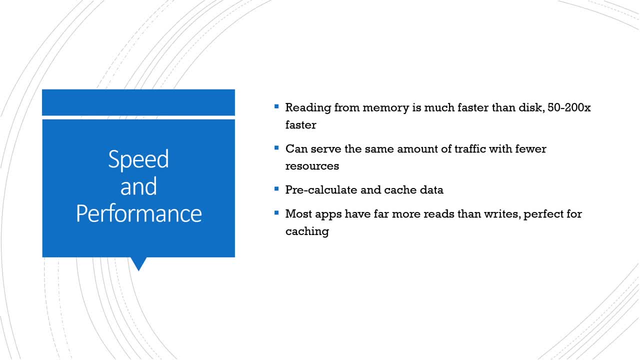 really improve performance that way. another big benefit is that most apps have far more reads than writes, which is perfect for caching. so again, if you think of something like twitter, where a single written tweet, so you write a tweet to a database, it's possible that that single tweet 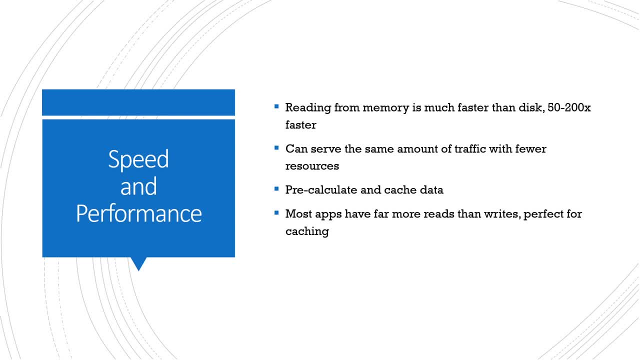 will be read thousands or, for a bigger account, millions of times. so instead of having for every one of those reads going to the database millions of times, you can put that into cache and it just gets served directly from there instead, which will really help the performance of your application. 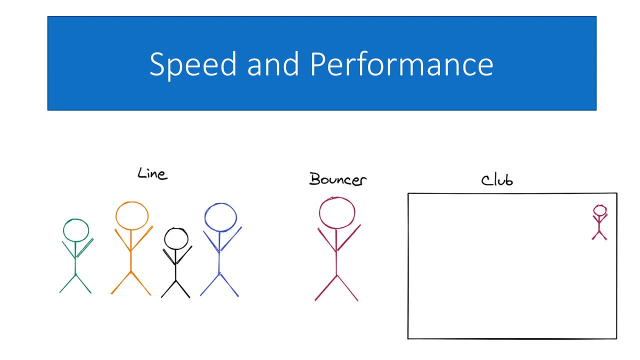 take a look at a real world example of how this kind of works and how it can make more sense to you maybe, which would be: we're going to use a club with a bouncer and people who want to get in. so this is our club, is essentially our application inside. here we have the owner, who would be kind. 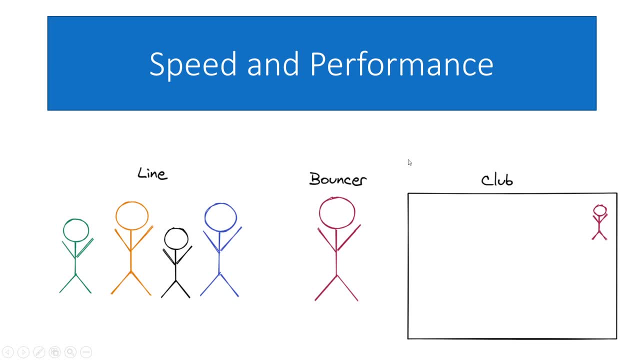 of the database. our bouncer has the password to get inside and we have our people who want to get in here. they're like clients or users in a web application. so one way to do it- the smart way- that would be like caching. the bouncer has the password in memory, literally, in this case, in his memory. 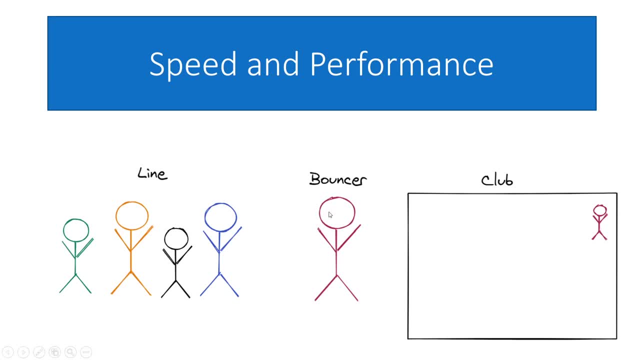 and all these people they ask. they say, hey, this is the password. he says that's right, lets him in. that would be very fast. the other way is, theoretically he could. every time somebody gives him the password, he walks into the club, goes all the way to the back room, asks the boss, or in this: 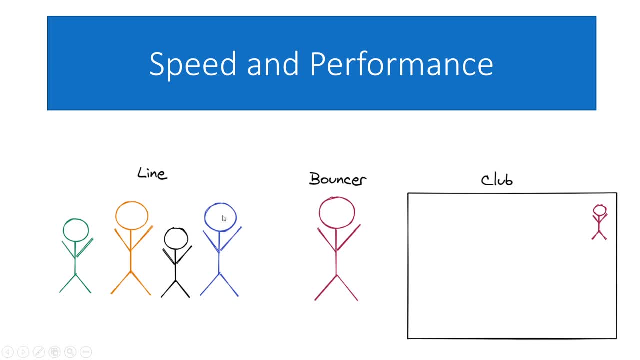 case, the database- hey, is this the right password? comes back, tells them yes or no. that would obviously take many times more time than it would take for the bouncer to be able to get in there. so there are things that a lot of people can do, and that's what we want to think about now. 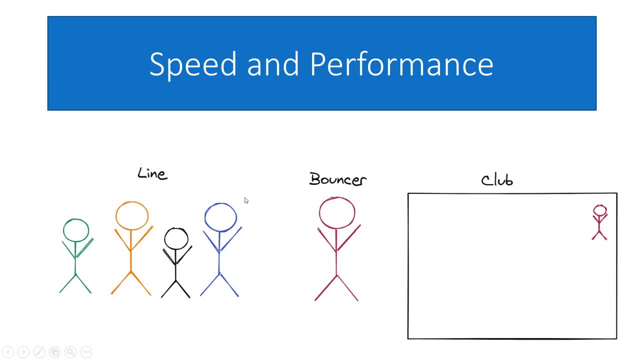 but not just just by getting in there to the back of the person real time, but maybe doing a better job with having a little bit of privacy. so maybe only segunda três seeds is the one there. but like a lot of times, I think the launch of information works better when you get online and it just gets so much easier because sometimes 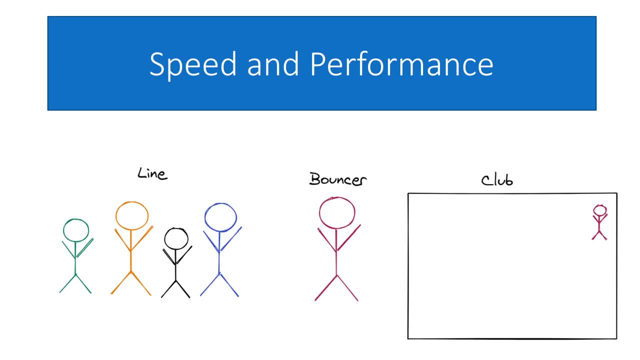 people might be good, and it's just not going to work unless you're typically using multiple services like others or, on the other hand, I'm a huge aa fan, so having that in mind is is really benefit to the application relationship as well. weren't you just say: I'm going to change what was? 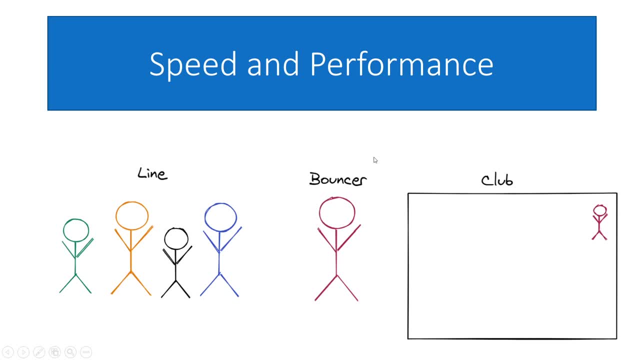 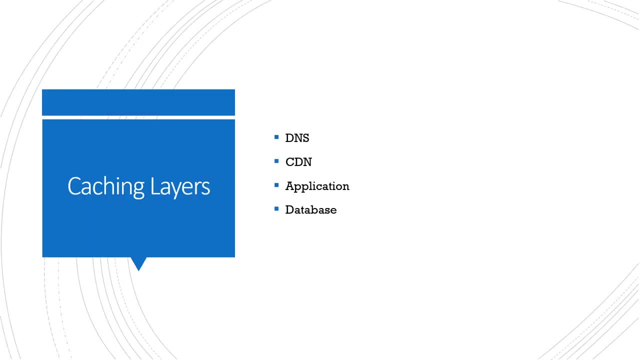 database. for that same information, you're much better off storing it up front in your cache, and that's just a better way to build your systems. also, use caching at multiple different layers, not just in front of your database, the main ones being DNS, content distribution network, CDNs, your application and like. 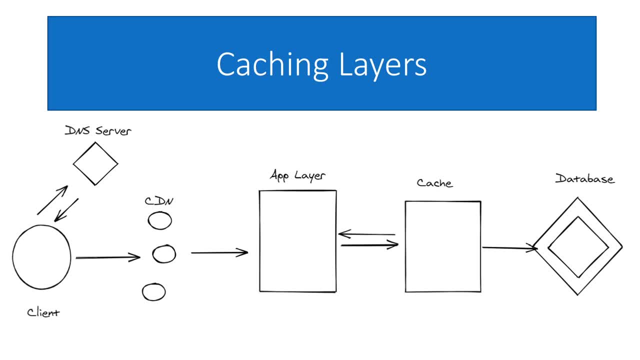 we've looked at the database itself. here's a diagram showing this. so you have your clients. when you type in like googlecom, for example, you don't actually go to Google. you go to an IP address and to get that you usually have to access it from a DNS server. so instead of going back and forth every 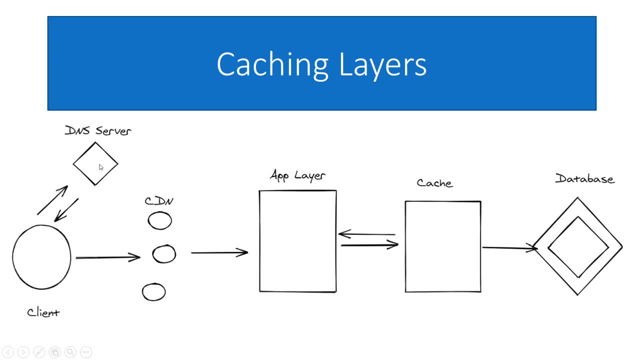 time to find the proper IP address. it usually makes that request once and then it stores it on the client so you can go to it directly. so that's one layer of caching. you then have content distribution networks, that's. if you've heard about cloudflare, you're probably familiar with it, because every few 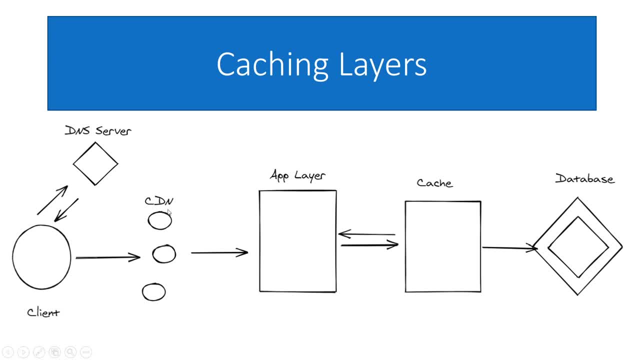 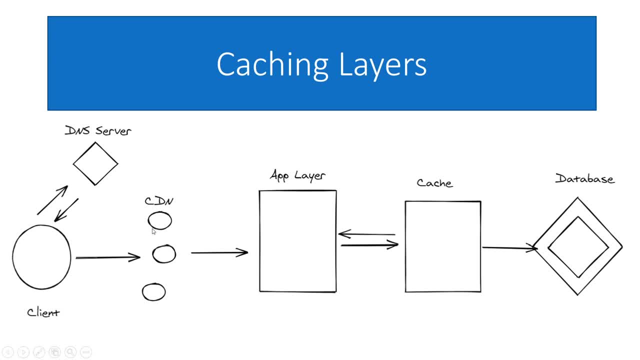 internet will go down, so a lot of websites use. internet will go down, so a lot of websites use these. and this is another way you can these, and this is another way you can these and this is another way you can store up front instead of having to get. 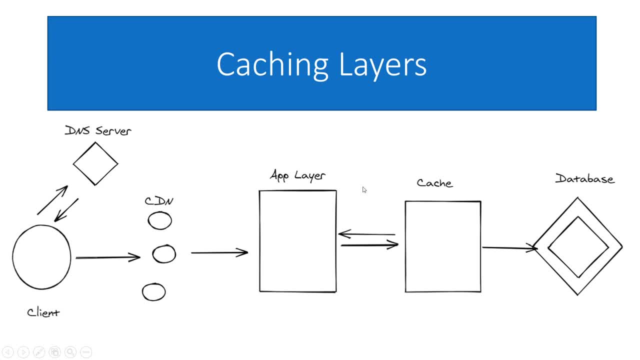 store up front instead of having to get store up front, instead of having to get static files- usually like pictures, and static files usually like pictures, and static files usually like pictures and videos. instead of serving them from your videos, instead of serving them from your videos, instead of serving them from your own infrastructure, you can push them to. 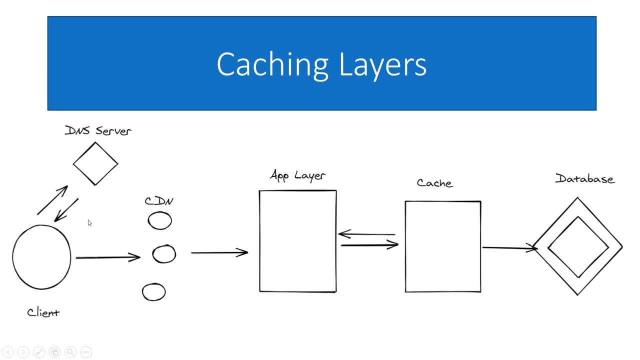 own infrastructure. you can push them to own infrastructure. you can push them to these CDNs and that will boost these CDNs and that will boost these CDNs and that will boost performance. they'll serve them back performance. they'll serve them back performance. they'll serve them back directly. then have your app layer and 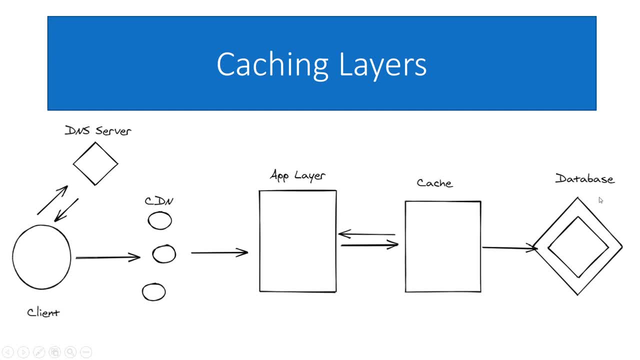 directly then have your app layer and directly then have your app layer and, like we said earlier, your cache here and, like we said earlier, your cache here and, like we said earlier, your cache here and most databases also have internally. we most databases also have internally. we most databases also have internally. we have inside frequently access data. 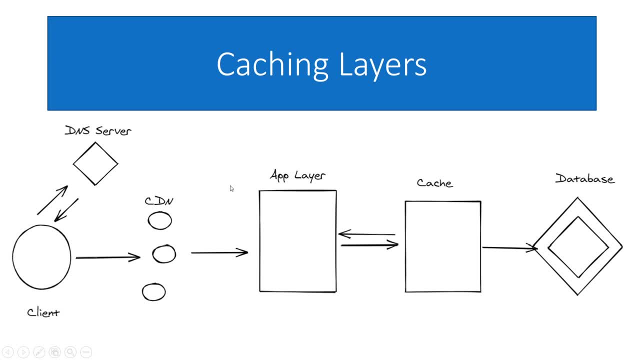 have inside frequently access data. have inside frequently access data- they'll automatically cache that as well. they'll automatically cache that as well. they'll automatically cache that as well. so you have multiple layers all across. so you have multiple layers all across. so you have multiple layers all across your application where it takes. 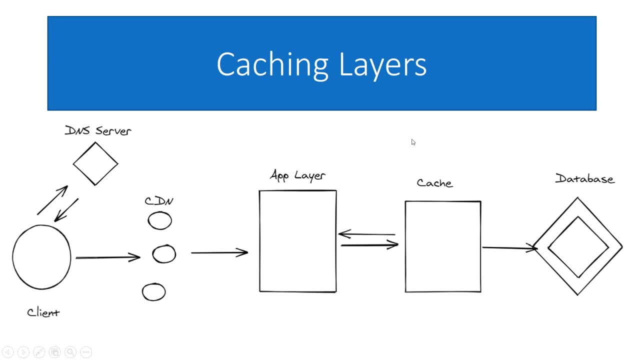 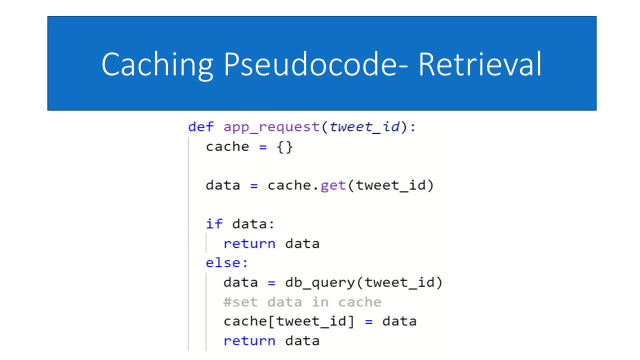 your application where it takes your application, where it takes advantages of the speed boost, from advantages of the speed boost, from advantages of the speed boost, from utilizing caching. here's some pseudocode utilizing caching. here's some pseudocode utilizing caching. here's some pseudocode with Python, kind of simulating how you 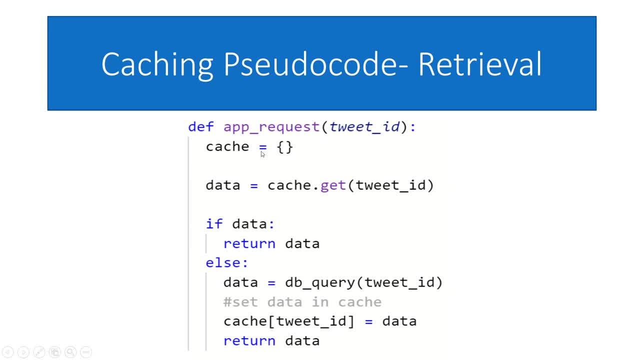 with Python kind of simulating how you with Python kind of simulating how you use a cache in your application. in this, use a cache in your application. in this, use a cache in your application. in this case we're just using a built-in case we're just using a built-in. 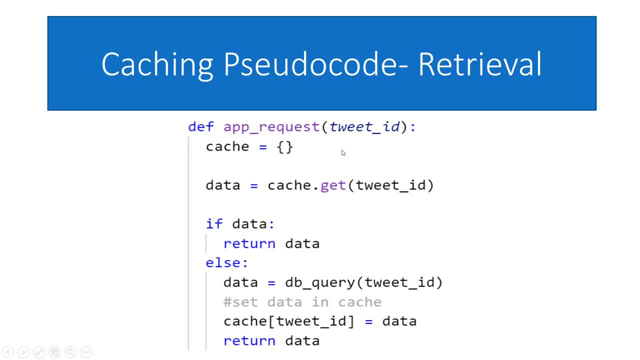 case, we're just using a built-in dictionary or hash table to simulate dictionary or hash table. to simulate dictionary or hash table. to simulate this. because that's what a cache really this. because that's what a cache really this. because that's what a cache really is, like readies or memcached it's. 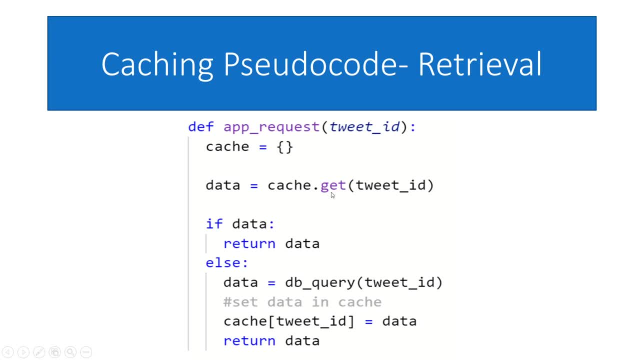 is like readies or memcached. it's is like readies or memcached. it's essentially just a giant in-memory hash, essentially just a giant in-memory hash, essentially just a giant in-memory hash ID. if that returns data from the cache ID. if that returns data from the cache. 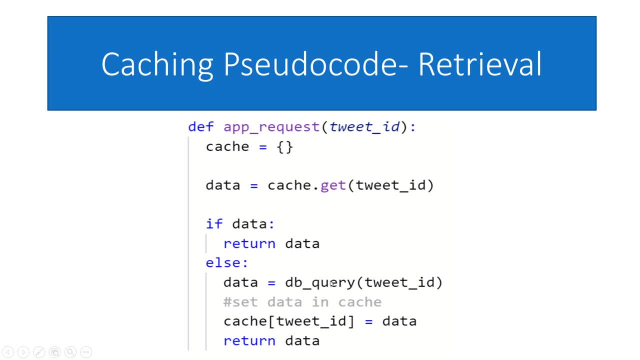 ID. if that returns data from the cache, we'd return that directly. otherwise we we'd return that directly. otherwise we we'd return that directly. otherwise we do a database query with that ID. we do a database query with that ID. we do a database query with that ID. we return the data. we set that into the. 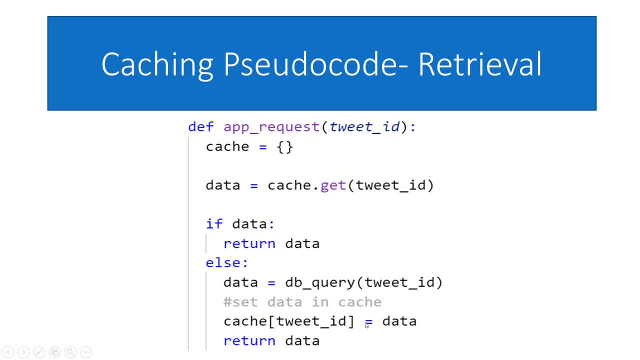 return the data. we set that into the return the data. we set that into the cache, and then we also return it. so this cache, and then we also return it. so this cache, and then we also return it. so this time, when we do this, the next time a. 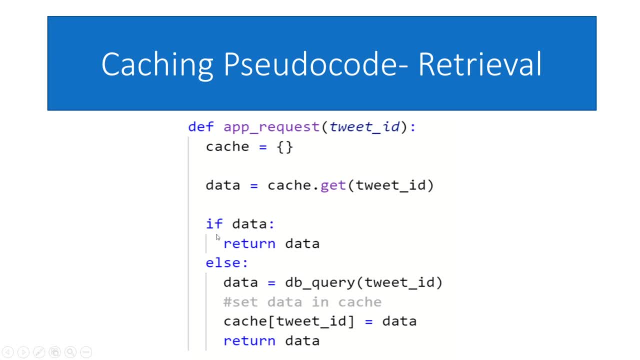 time when we do this, the next time, a time when we do this, the next time a user requests that same tweet, it'll hit user requests that same tweet. it'll hit user requests that same tweet. it'll hit here and it will return. so we don't. 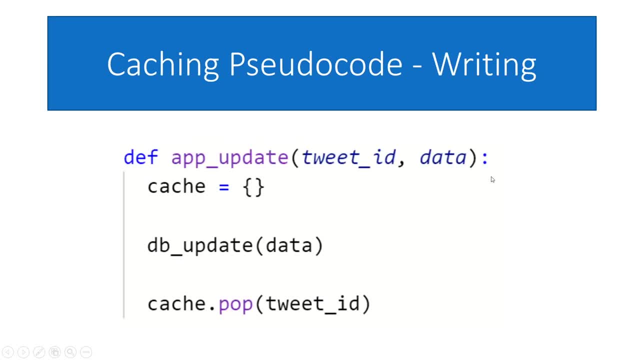 here and it will return. so we don't here and it will return. so we don't have to make that database query for, have to make that database query for, have to make that database query for rights. we've got a similar setup where rights. we've got a similar setup where. 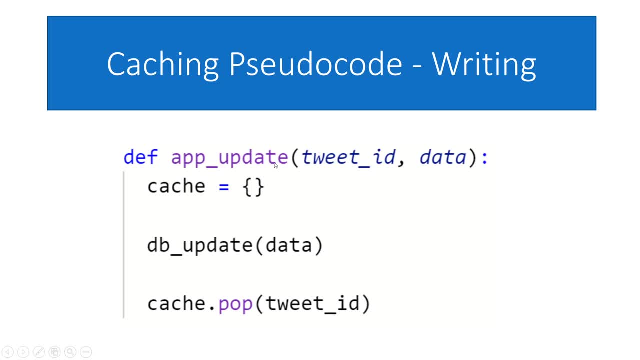 rights. we've got a similar setup where it's just caching. so in this case, if it's just caching, so in this case, if it's just caching, so in this case, if we're updating a value, we go to our. we're updating a value, we go to our. 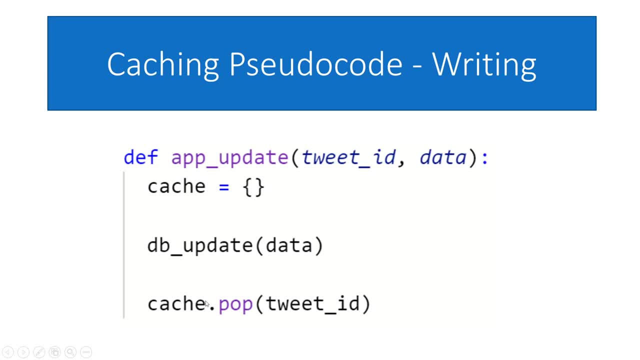 we're updating a value, we go to our database, we update the tweet and if the database, we update the tweet. and if the database, we update the tweet. and if the tweet is already in the cache, we want tweet is already in the cache. we want tweet is already in the cache. we want to make sure we remove it so that we 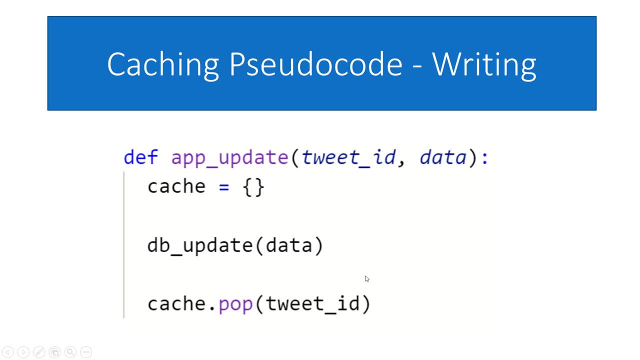 to make sure we remove it, so that we to make sure we remove it, so that we don't have an issue with what is called, don't have an issue with what is called, don't have an issue with what is called stale data, and we'll go over that a. 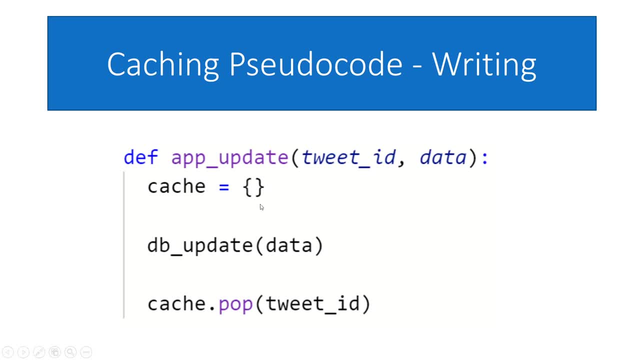 stale data and we'll go over that. a stale data, and we'll go over that a little bit later, but what that is is that little bit later. but what that is is that little bit later. but what that is is that we don't want users seeing the old. 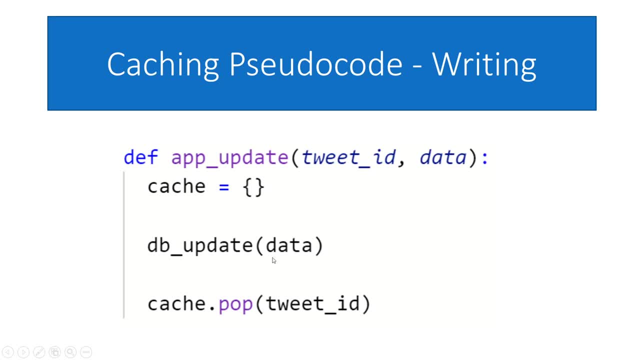 we don't want users seeing the old. we don't want users seeing the old version of the tweet or whatever data we version of the tweet, or whatever data- we version of the tweet or whatever data we just updated. so we remove it from the just updated. so we remove it from the. 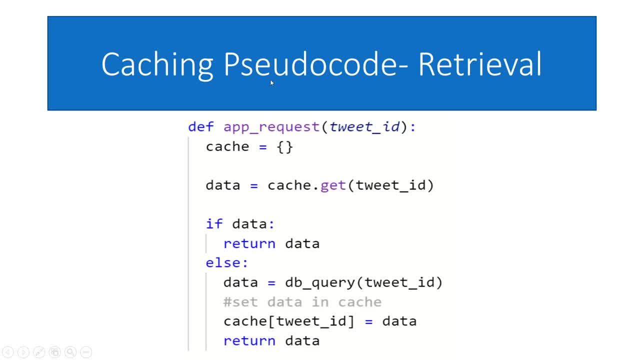 just updated so we remove it from the cache, so that the next request if we go cache, so that the next request if we go cache, so that the next request if we go back, it will re-grab that from the back, it will re-grab that from the. 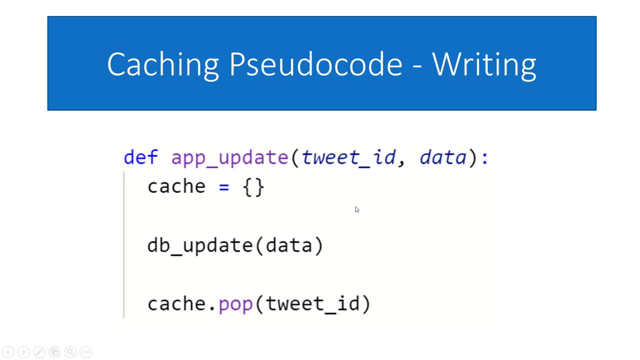 back, it will re-grab that from the database, and that way we're not getting database. and that way we're not getting database. and that way we're not getting old data for our users. building off of old data for our users, building off of old data for our users, building off of simple caching, we have what's known as. 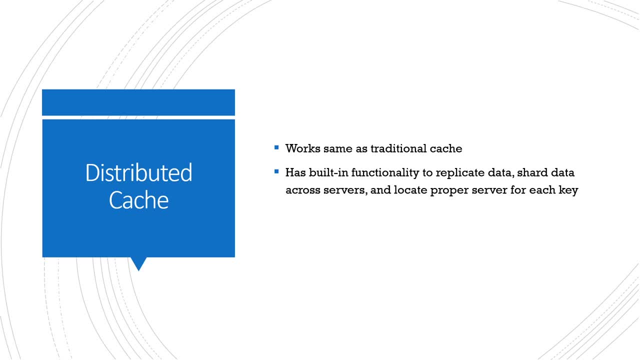 simple caching. we have what's known as simple caching. we have what's known as distributed cache, which it works. the distributed cache which it works. the distributed cache which it works the same way, but it has built-in same way. but it has built-in same way, but it has built-in functionality to replicate the data. 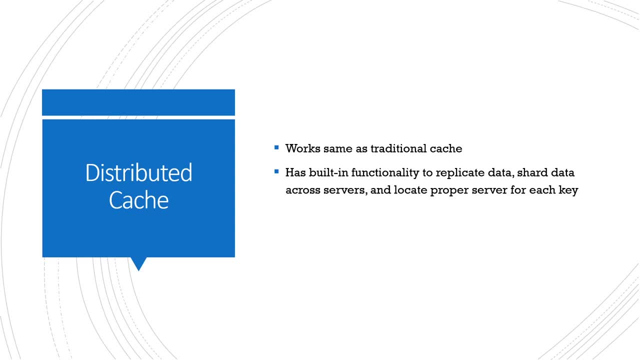 functionality to replicate the data functionality to replicate the data sharded across multiple servers, if our sharded across multiple servers, if our sharded across multiple servers, if our amount of data is too big for a single amount of data is too big for a single amount of data is too big for a single server, and then locate the proper server. 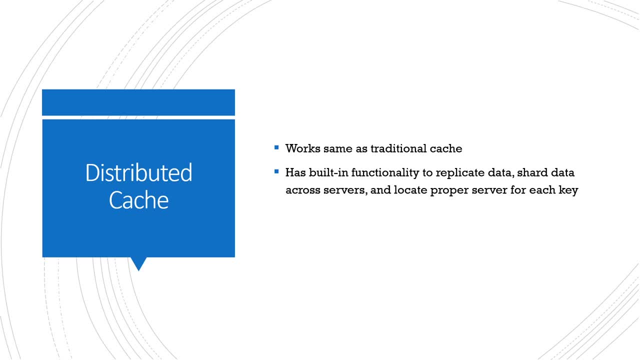 server and then locate the proper server server and then locate the proper server to find for each key that we're using, to find for each key that we're using, to find for each key that we're using. the main reason you do this is that at the main reason you do this is that at 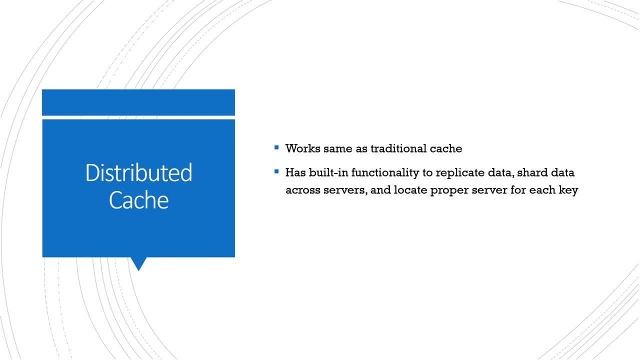 the main reason you do this is that at scale, you don't want your entire system scale. you don't want your entire system scale. you don't want your entire system to break down just because your single to break down, just because your single to break down, just because your single cache server goes down. so you want some. 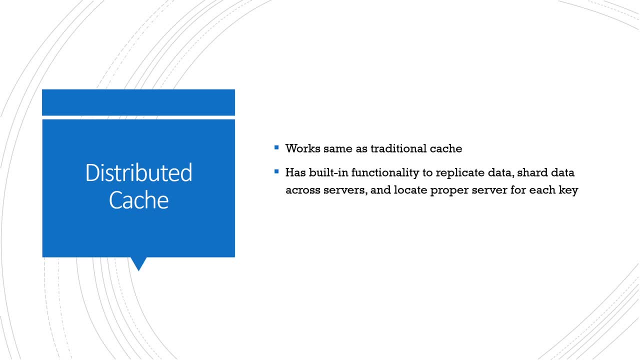 cache server goes down, so you want some cache server goes down, so you want some replication and stuff like that, so that replication and stuff like that, so that replication and stuff like that, so that your system is more reliable. your system is more reliable, your system is more reliable. you can visualize it here, so you'd have 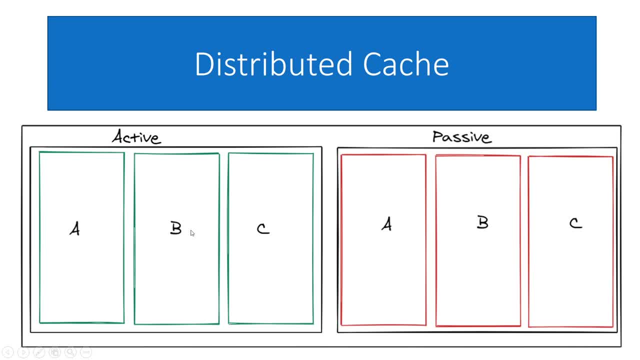 you can visualize it here, so you'd have- you can visualize it here, so you'd have a active server. you have multiple a active server. you have multiple a active server. you have multiple with different keys, so you have abc and with different keys, so you have abc and. 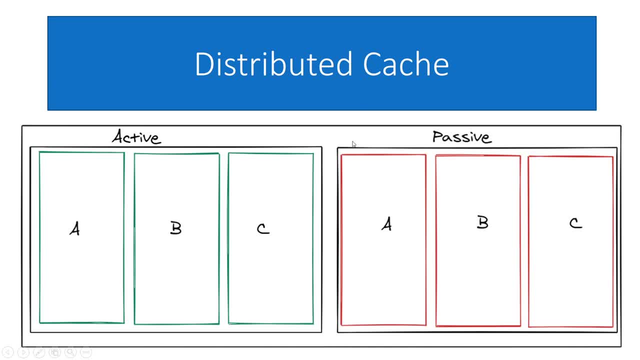 with different keys. so you have abc and you also want sitting here, your passive. you also want sitting here, your passive. you also want sitting here, your passive. so if one of these goes down, your, so if one of these goes down, your. so if one of these goes down, your application will be able to detect that. 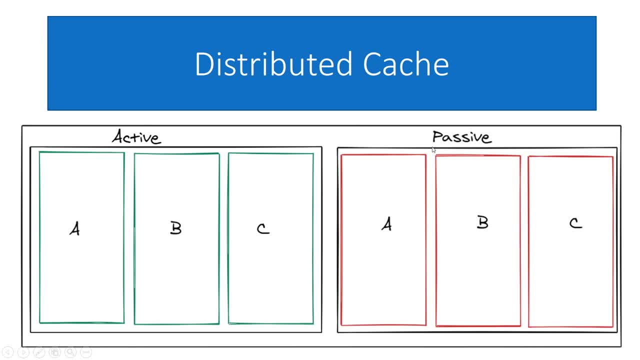 application will be able to detect that and it will reroute to your passive server, which is now the active one. the thing it might seem wasteful, because what you want is basically: these are going to be identical, they're going to be in communication and have the same amount of data, but these 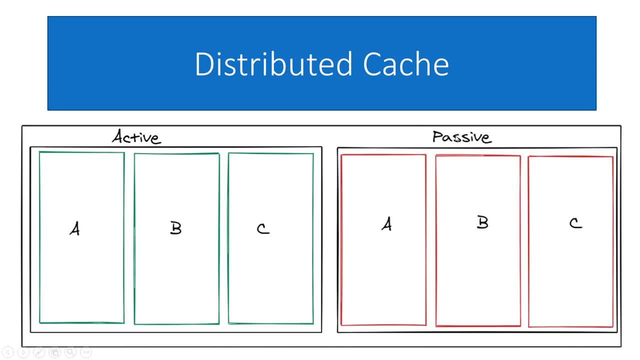 under ideal conditions will never actually do anything. best case scenario is you never have to use your backups. but the reason you have this is that if this cache goes down and all of a sudden all those queries are going to your database, you're going to have big issues. 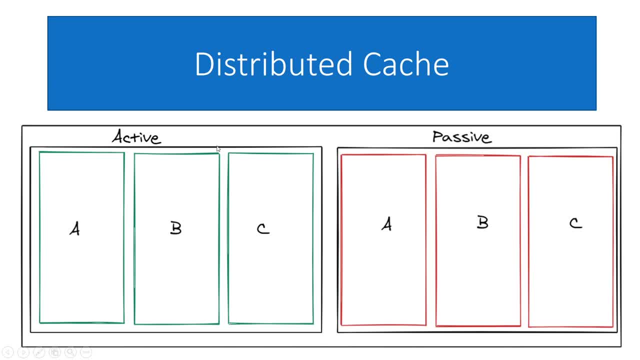 because your system is built assuming that, let's say, 90 some percent of your requests are going to be served from cash. so if these goes down all of a sudden, your database are going to be overwhelmed by that amount of traffic. so you have these backups and that's what that's going to help with. 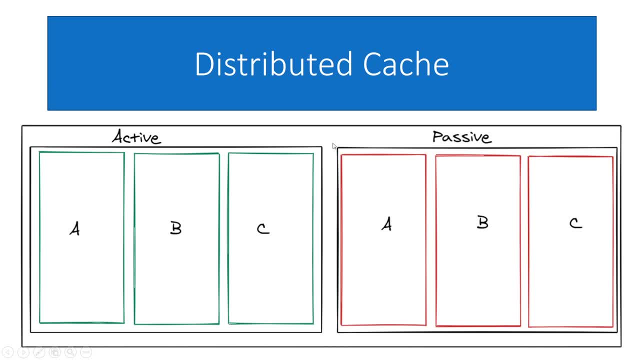 another big thing is that something facebook wrote about early in their company history was that they had big issues with they didn't have this pre. they called it a warm-up, where they didn't have this data pre put into these caches so they'd spin up this would go. 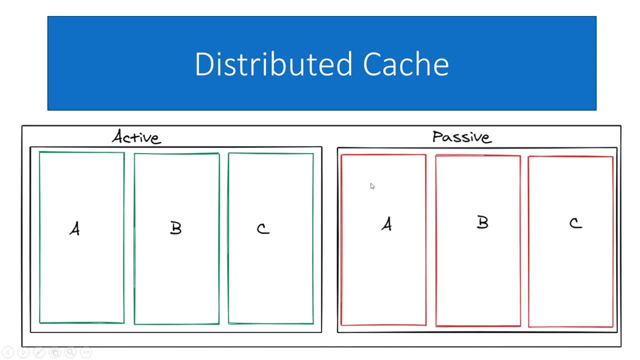 down, they'd automatically spin up a new one. but the issue was that they'd have a 100 cash miss initially, so everything would go straight through it because it's empty, and then it would have to fill up gradually. so one of their solutions this problem was they would do what they call a warm 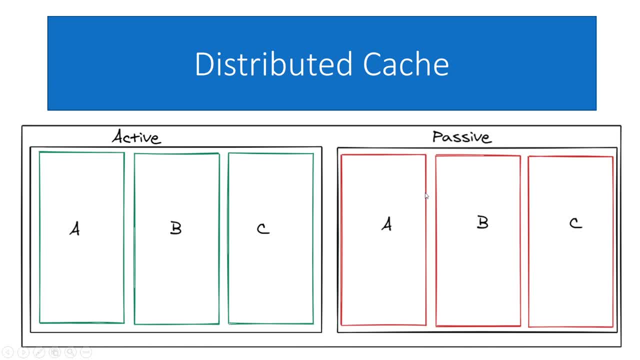 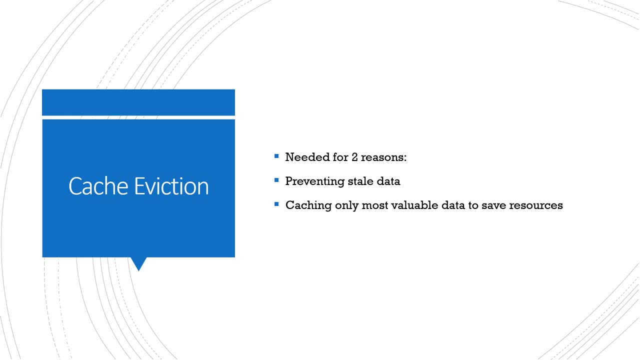 up and, before they even brought these online and made them available, they would pre-query the database and fill up these caches so that they didn't have that issue. moving on, a key concept is cache eviction. we need this for two reasons, which is like we talked about. 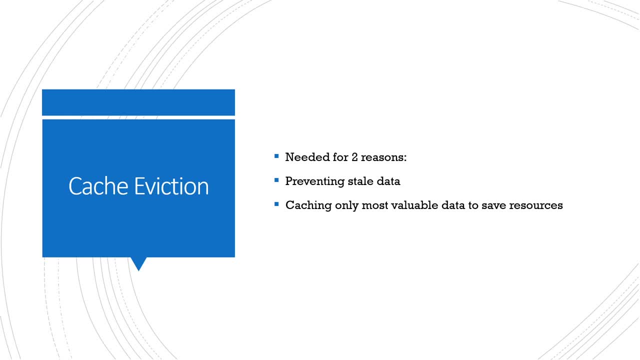 earlier. we want to prevent stale data. we don't want something sitting in cache for too long because if it's updated, we don't want um out of date stuff being served the user. we don't want out of date stuff being served the user. we don't want out of date stuff being served the user. 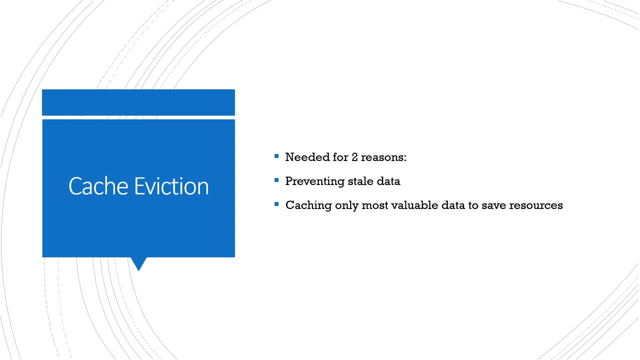 users. We also want to only cache the most valuable data to save money and resources. There's a lot of stuff in your database that might never or very rarely be requested, so it doesn't really make sense to store that stuff and cache, because it's just kind of. 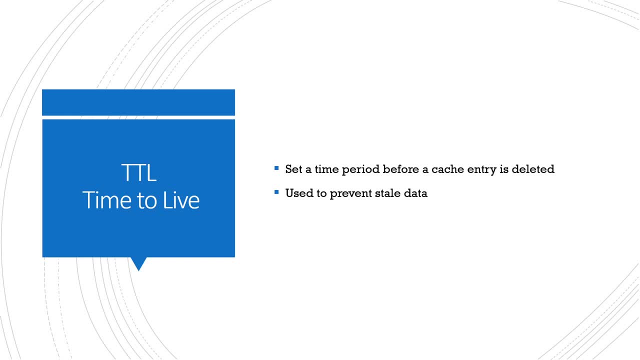 a waste. So the first major thing is TTL: time to live. This is where you could set a time period before cache entry is deleted automatically. This is mainly used to prevent stale data, and the time that you set can depend on how essential it is for data to be fresh. So in some cases- let's say a blog post- it's very rarely going to be updated, so you could probably set a longer cache time. Same thing with something like tweet counts, like if you have a tweet and you have a certain amount of likes, it doesn't need to be immediately updated If there's a few seconds or even. 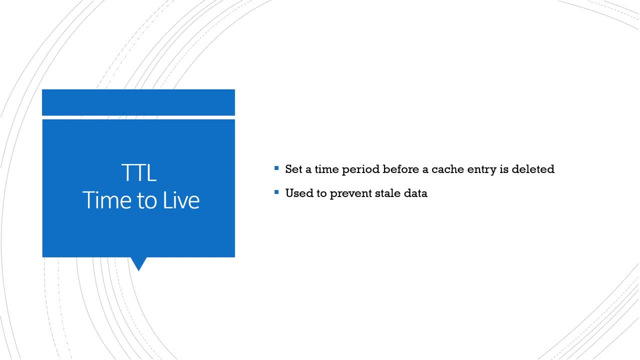 a minute where you let that serve stale data. it's not a huge deal. It's not like there's people's lives depending on the exact, accurate count on the number of likes on a tweet. In other cases, for something that's very important, like something related to healthcare, where it's somebody's heartbeat count or their breathing rate that you probably don't even want to cache. You want it to be constant live data so that you don't have a delay, because that could literally kill somebody. So you don't want that. The TTL time: it kind of just depends. 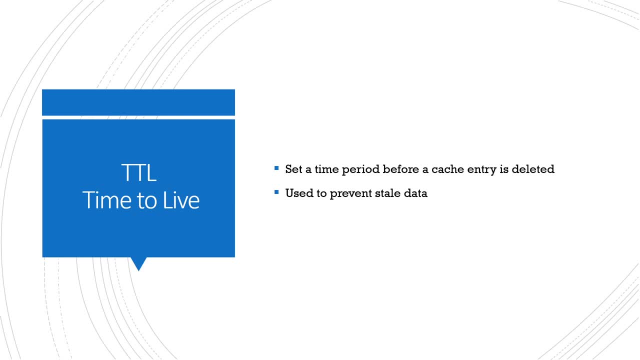 on what kind of data you're working with. So LRU and LFU are two other strategies. These have less to do with preventing stale data and more to do with trying to keep our most requested data in our cache. So least recently used is: once our cache is full, we can't obviously add any more keys, so we have to choose what. 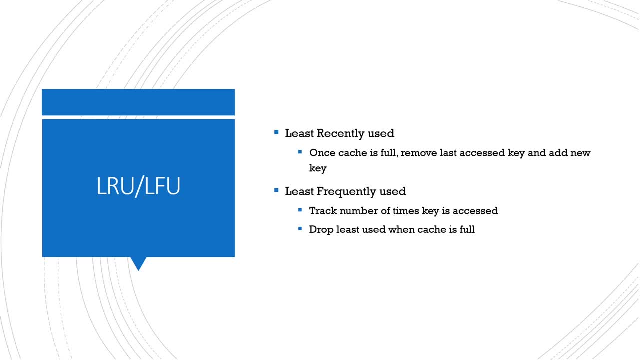 do we get rid of So this strategy? what happens is whatever hasn't been accessed, or what was last accessed, latest, we get rid of that because it's not being as frequently requested, so it's less risky for us to drop that. The other one is: 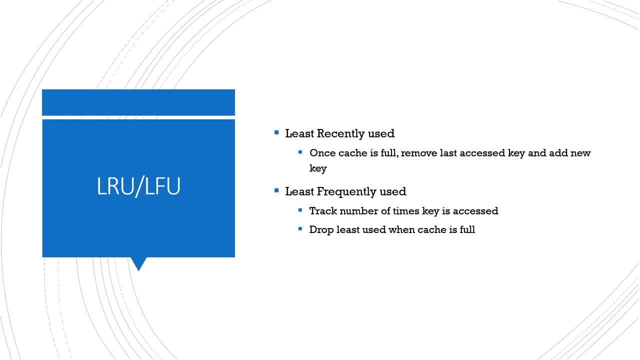 kind of similar same concept, which is it tracks the number of times a key has been accessed and once our table is full it will get rid of whichever one during that time period has been the least requested. So the concept here is that we want to make sure that highly accessed data- we keep that in cache Less requested. 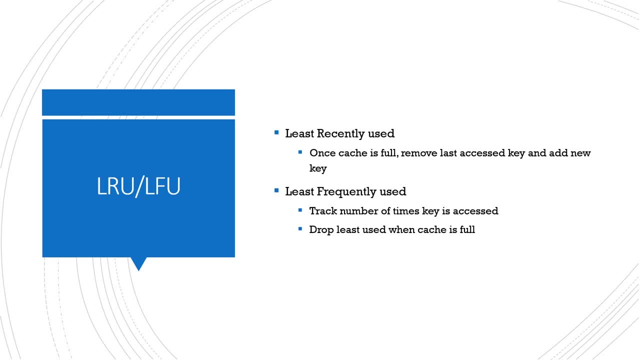 stuff. it's a little bit safer to request that from the database. Some examples of this in practice: Let's keep working with Twitter. Let's say we have two different tweets, So in our database they're the same size, but there's a big difference between a tweet from: 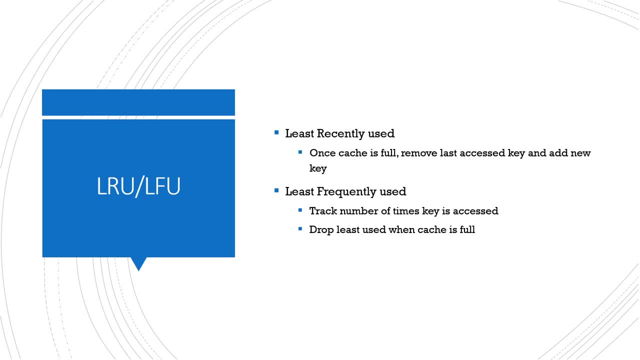 2012, From a small account with 10 followers, verse a tweet that was just created by an, an account with millions of followers. The one from 2012 or whatever year it was, barely is ever going to get requested, So it's not a big deal if, once a month, somebody requests that from the. 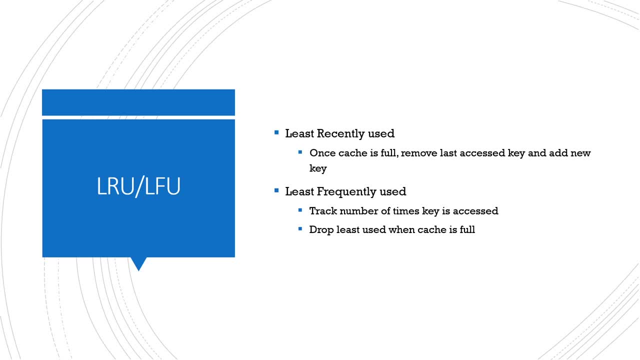 database. On the other hand, the recent tweet is going to be wanted. There's going to be read requests millions of times for it, So we want that in our cache so that our database isn't getting destroyed by all those requests. Another example related to cache eviction: 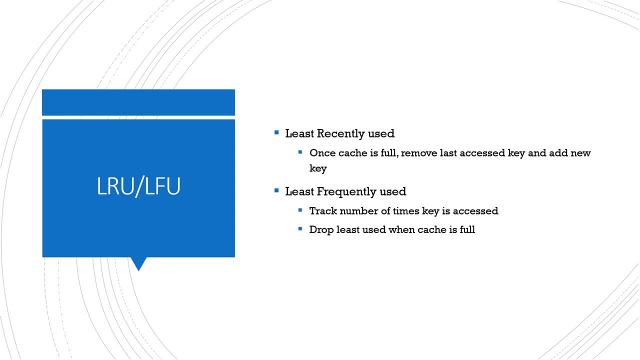 is from a Facebook case study. They called it the thundering herd problem. So they'd have a situation where some user would update a post, like a popular user updates a post. they dump that from cache When you have thousands of requests coming at the same time. 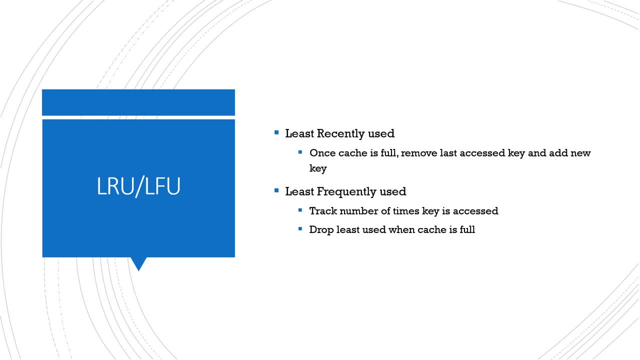 when we looked at our pseudocode we talked about on the second read request after we updated, they'd just refresh it. But the problem is when you have thousands or tens of thousands of requests coming at the same time, you're going to have thousands of requests coming at the same. 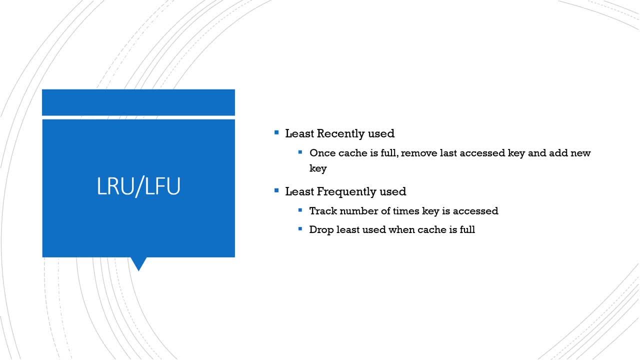 time. So what would happen is that a bunch of them at the same time would go straight through the cache and still make that read request, which would cause tons of issues from their database. So their solution to this issue at scale with cache eviction was that they would implement. 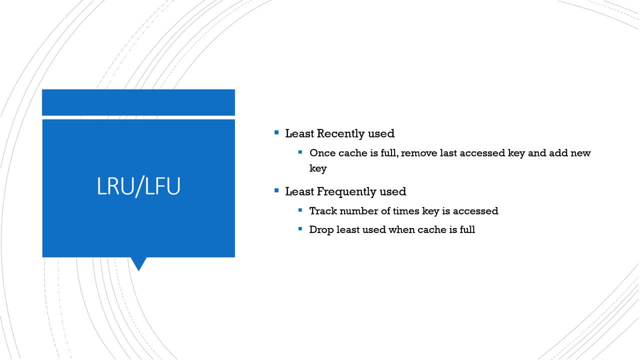 what's called a lease, So they'd have kind of like a backup cache that would still serve that old data while the cache updated in the background. So that's something you probably won't have to worry about. But if you have a cache that's not updated, you're going to have to update it, So that's. 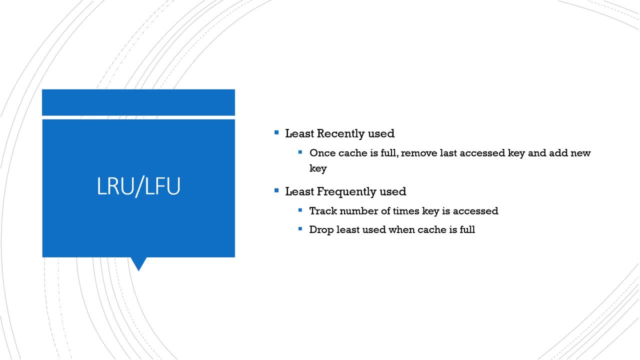 something you probably won't have to worry about, But it shows that at scale, stuff that you really don't even think about, like what would happen if I get thousands of requests during the split second or something updates and gets removed- Most applications don't have to worry about that. 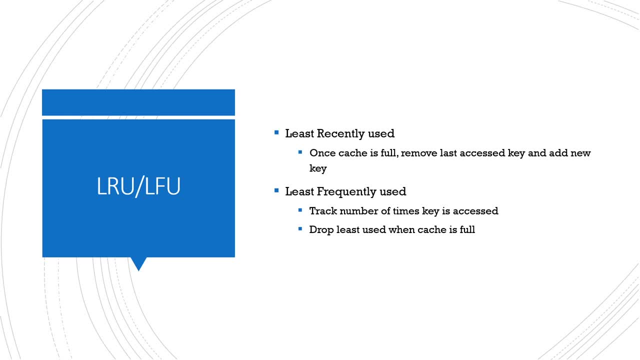 but it's kind of interesting that at large scale all sorts of things pop up that you'd never really think about. So there's a couple different caching strategies. The first one I showed with the pseudocode, is cache aside, and that's definitely the most common. 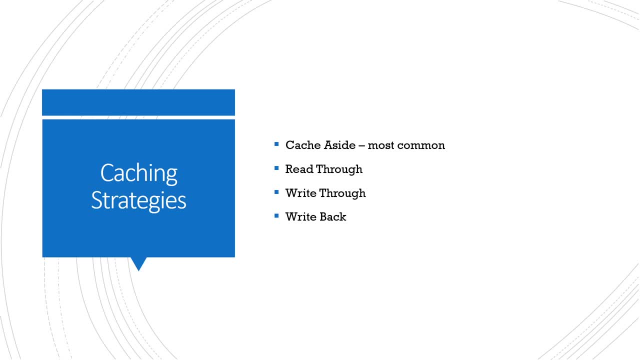 Write through and write back are kind of interesting because there'd be more for a write heavy application. So write through. what happens is that to increase the amount of writes the database can handle, the cache is actually updated before the database. What this does is it allows to maintain. 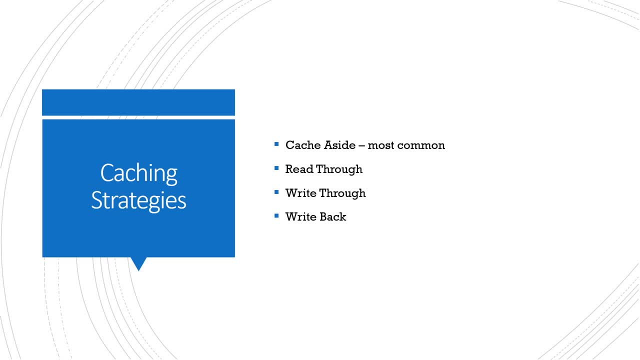 high consistency between your cache and your database, But as a result, it adds latency to whenever a user writes, So it's going to slow things down from that perspective. The write back strategy involves writing data directly to the cache, which is very fast. 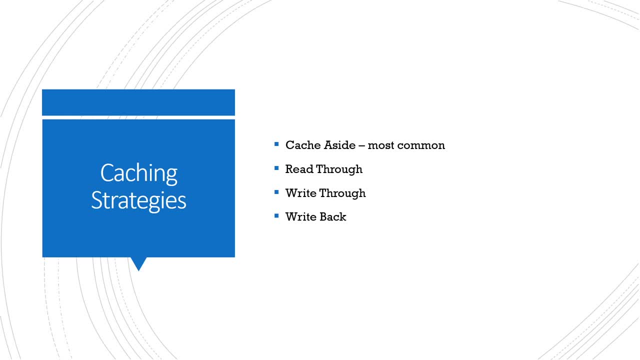 But a side effect of that is that if your cache fails before it can write that data to your database, you have an issue with data loss. So that's kind of a riskier strategy. But if you really need to scale writes for some reason and consistency isn't essential, that's one way to do. 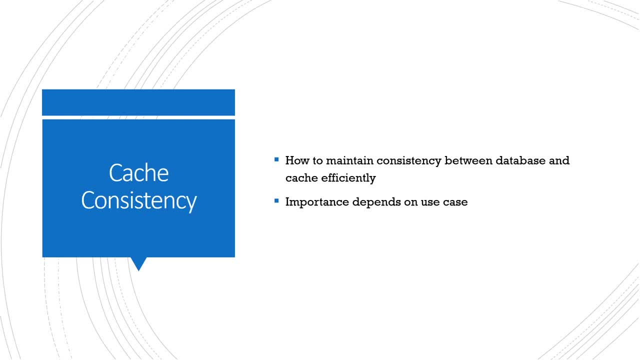 it. And finally, we have cache consistency, which I touched on earlier, And that's basically amounts to you want to make sure that your cache and your database are showing the same thing. The importance of that. if there's a slight delay, it depends on your use case. The biggest thing. 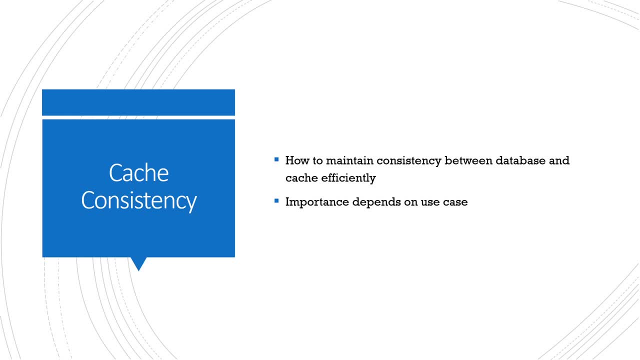 is that for writes, you want to make sure that the user who's writing data gets that fresh data immediately. Facebook wrote about that, where they had issues where users would update a post. maybe they made a typo or they accidentally posted something, So you want to make sure that. 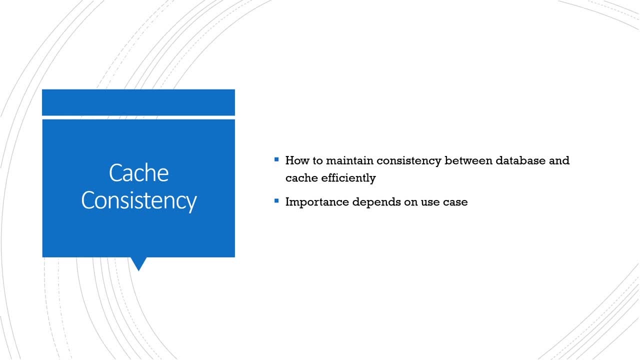 that's something they didn't mean to And they had a delay between when they would write it and when the user would see it. And the users were obviously getting upset because they wanted to immediately see that it was showing the new updated post rather than the old one, Because in some cases, if